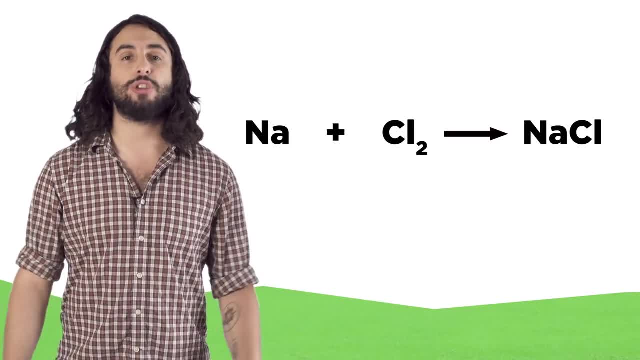 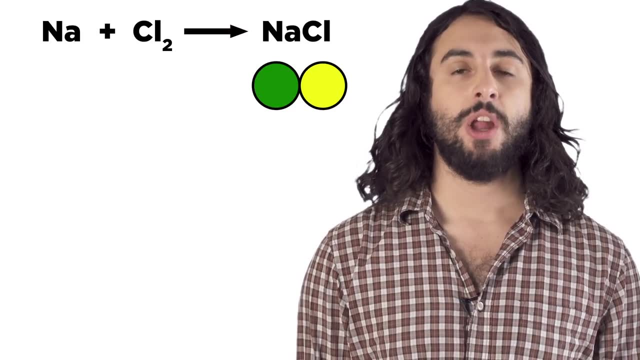 number of atoms on both sides, because atoms won't just appear or disappear, they all have to be accounted for. for example, in order to make one molecule of sodium chloride, we need one sodium atom and one chlorine atom. but chlorine gas molecules have two atoms of chlorine. 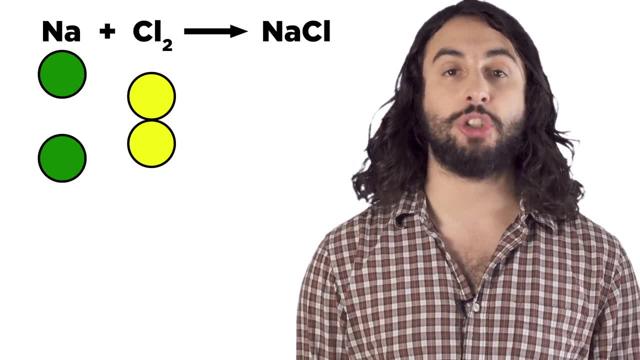 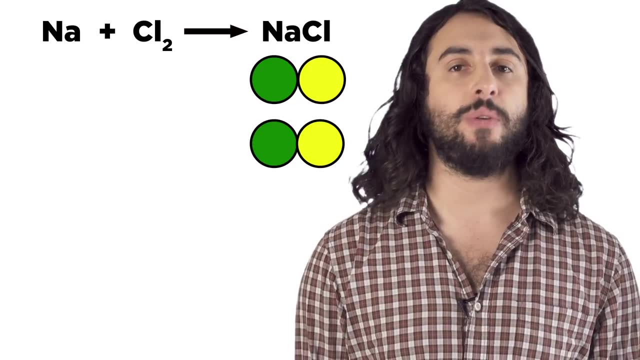 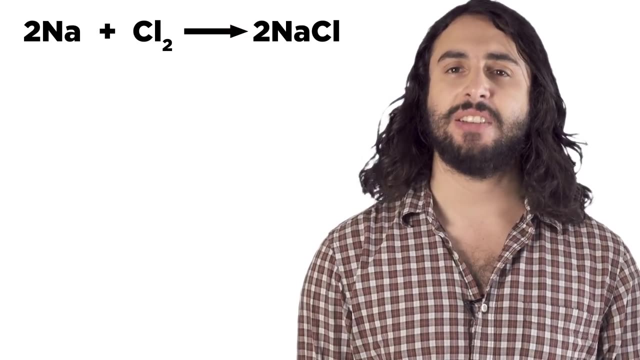 each. so one molecule of chlorine gas will react with two sodium atoms to give two molecules of sodium chloride. we need to include coefficients before each substance to indicate how many of each. we need to make the equation balanced. let's make the distinction that these subscripts tell us how many atoms of a 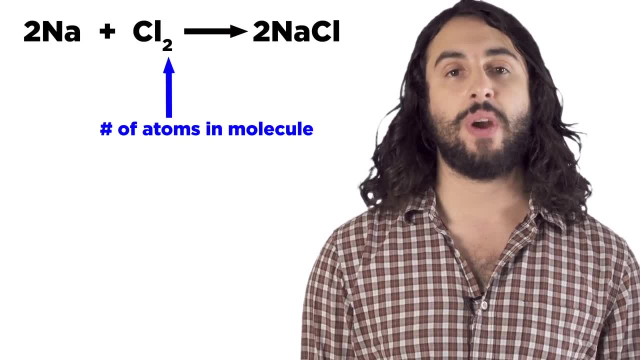 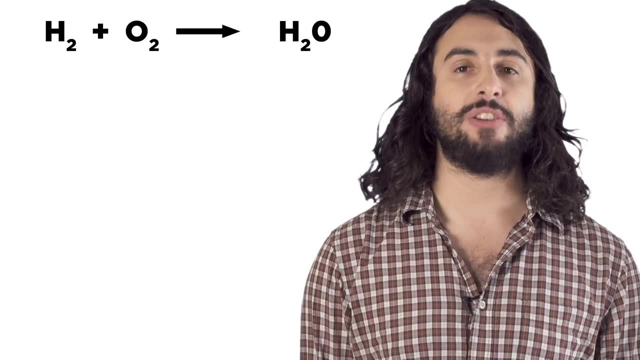 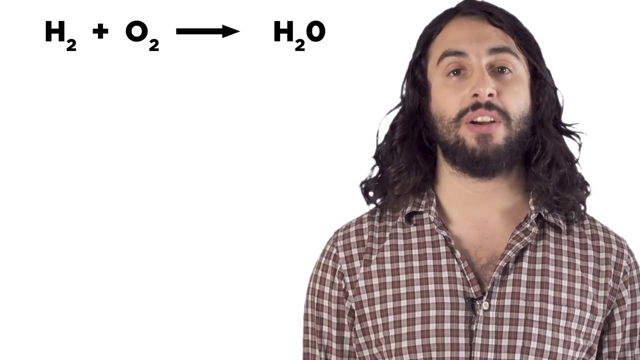 given element are in one molecule, whereas these coefficients tell us how many of that molecule there are in the reaction. where hydrogen gas and oxygen gas go to make water, we can see that the gases have two atoms each and water has two hydrogen atoms and one. 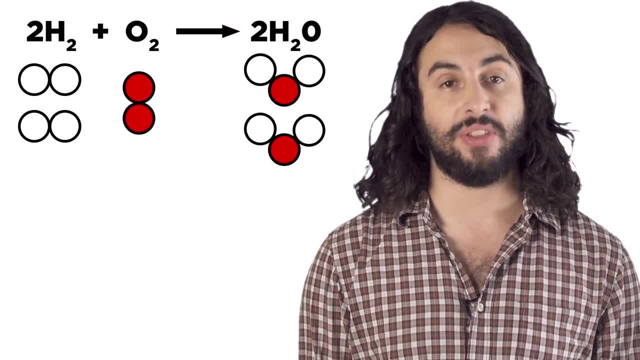 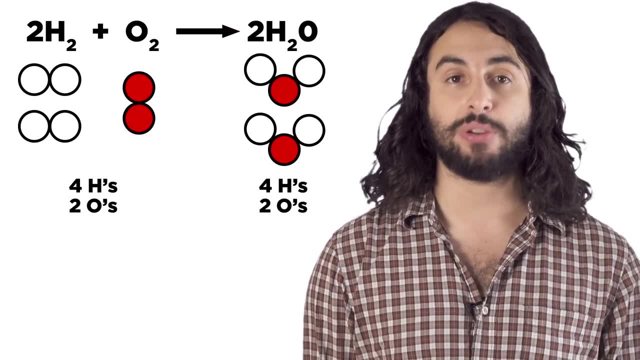 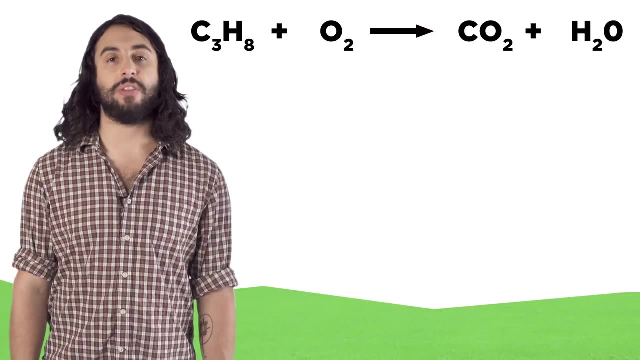 oxygen atom. we will need to combine these substances in this ratio to make this equation balanced. now there are the same number of hydrogen and oxygen atoms on both sides of the equation, even though they have rearranged their combinations. so if we have an unbalanced equation like this one that we need to. 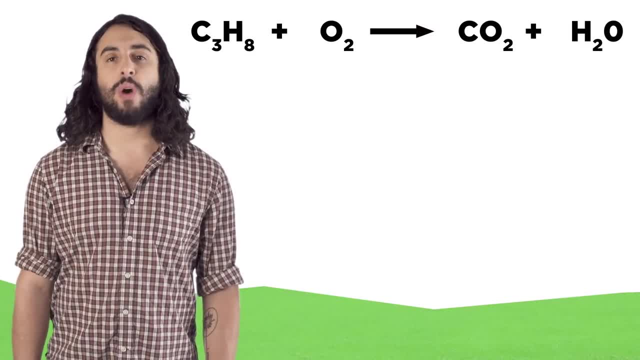 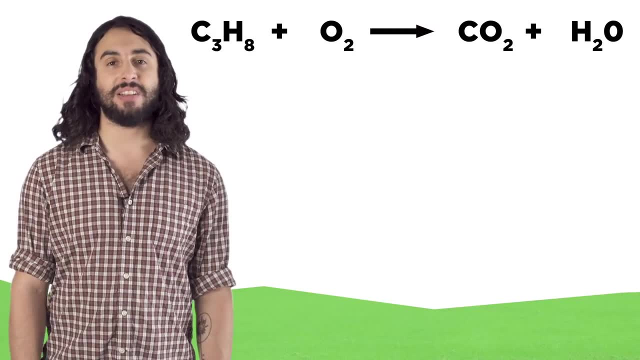 balance. there's an easy way to do it: we will balance things one element at a time. if an element exists by itself, do that one last. start with an element that is present in just one compound on each side. let's do carbon first on the left. 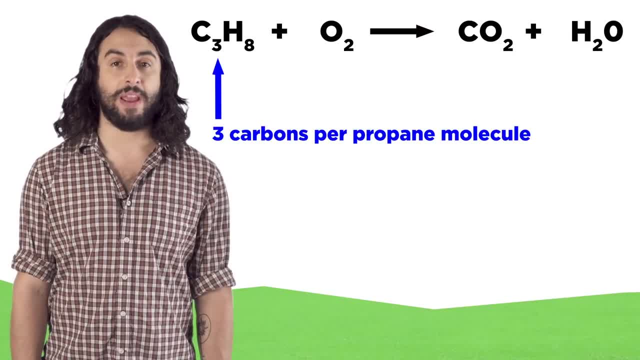 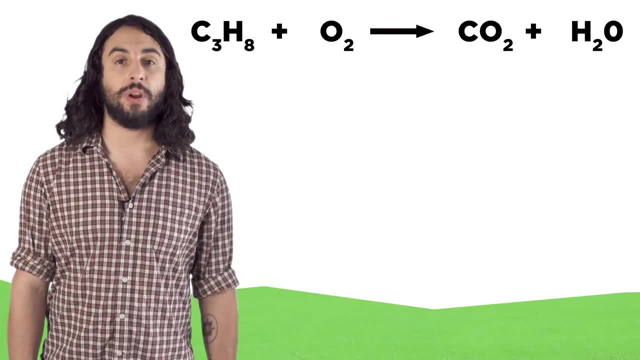 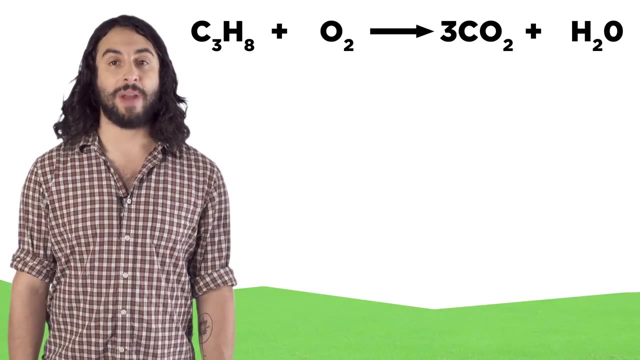 there are three carbon atoms for every molecule of propane and on the right there is just one for every molecule of carbon dioxide. so, according to the carbons, we are going to make three CO2s with every propane. let's put a three there. now the carbons are balanced: three carbon atoms on each. 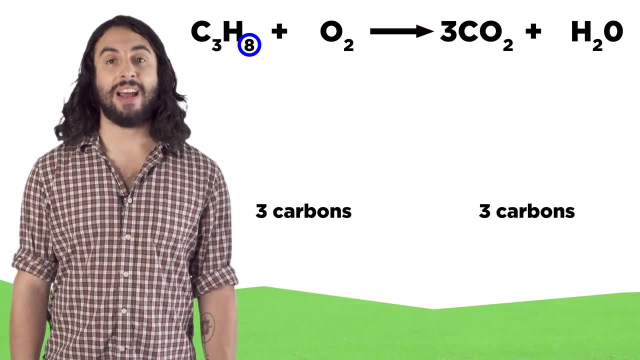 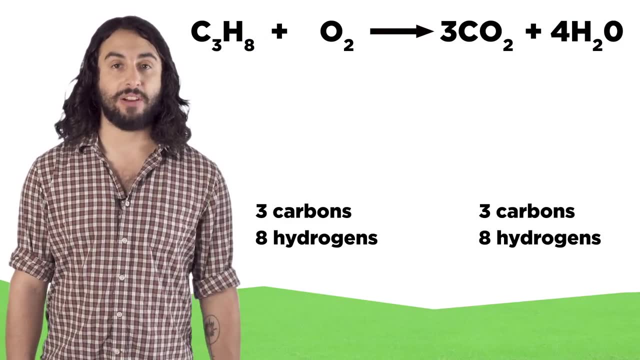 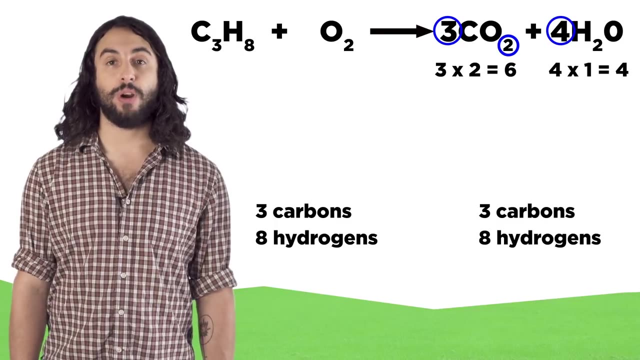 side. next let's do hydrogen. there's eight on the left and two on the right. that means we will make four waters with every propane. now hydrogen is balanced, eight on each side. last is oxygen. on the right there's six from CO2 and four.